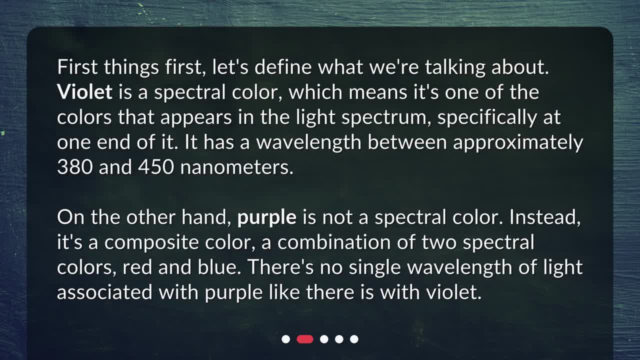 What are violet and purple? First things first, let's define what we're talking about. Violet is a spectral color, which means it's one of the colors that appears in the light spectrum, specifically at one end of it. It has a wavelength between approximately 380 and 450 nanometers. On the other hand, 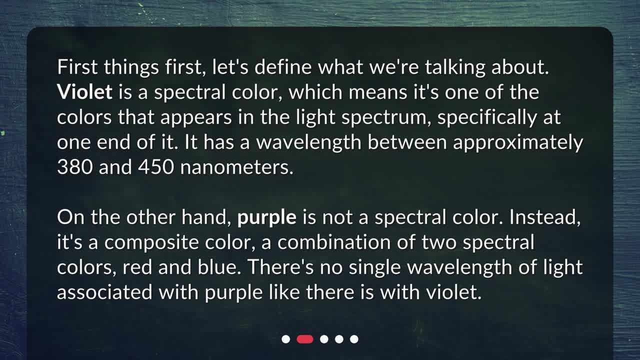 purple is not a spectral color. Instead, it's a composite color, a combination of two spectral colors: red and blue. There's no single wavelength of light associated with it, purple, like there is with violet. How do we perceive violet and purple? 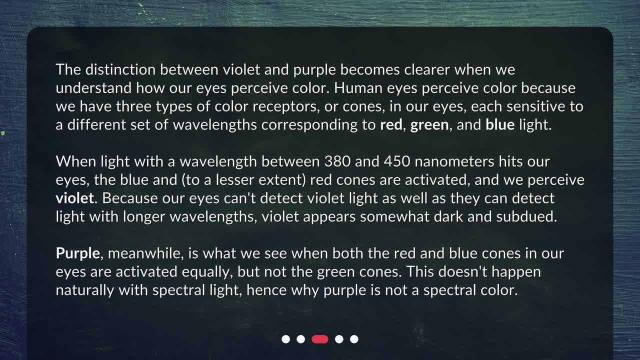 The distinction between violet and purple becomes clearer when we understand how our eyes perceive color. Human eyes perceive color because we have three types of color receptors or cones in our eyes, each sensitive to a different set of wavelengths corresponding to red, green and blue light. When light with a wavelength between 380 and 450 nanometers hits our eyes, 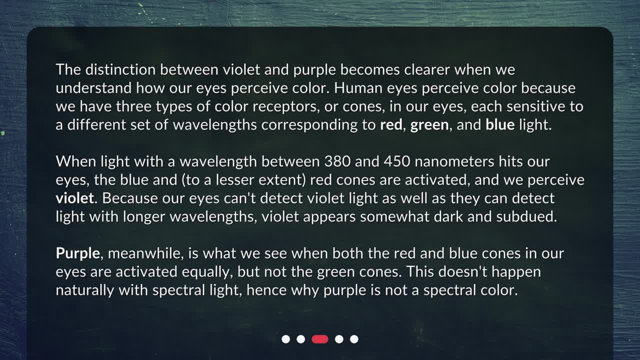 the blue and, to a lesser extent, red cones are activated and we perceive violet Because our eyes can't detect violet light as well as they can detect light with longer wavelengths. violet appears somewhat dark and subdued. Purple, meanwhile, is what we see when both the red and 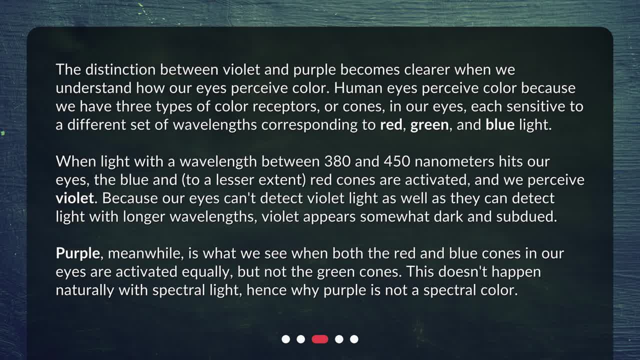 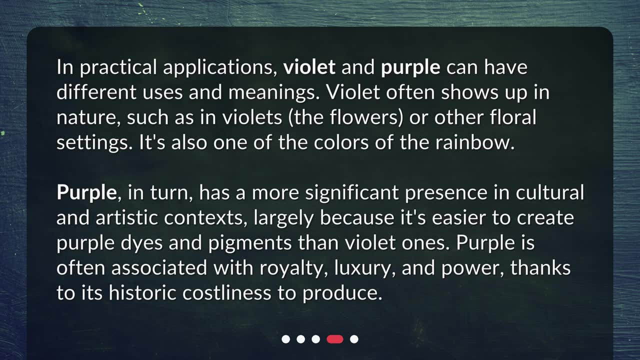 blue cones in our eyes are activated equally, but not the green cones. This doesn't happen naturally with spectral light, hence why purple is not a spectral color. Where do we use violet and purple In practical applications? violet and purple can have different uses and meanings. 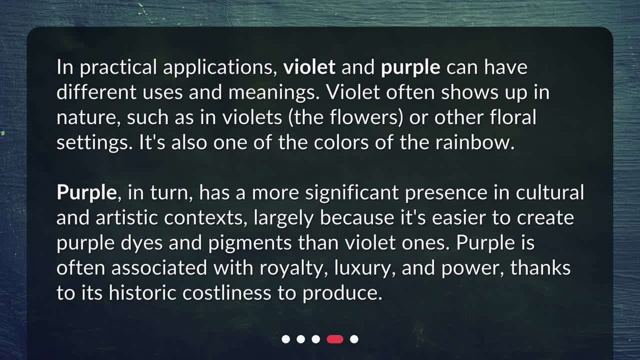 Violet often shows up in nature, such as in violets, the flowers or other floral settings. It's also one of the colors of the rainbow. Purple, in turn, has a more significant presence in cultural and artistic contexts, largely because it's easier to create purple dyes. 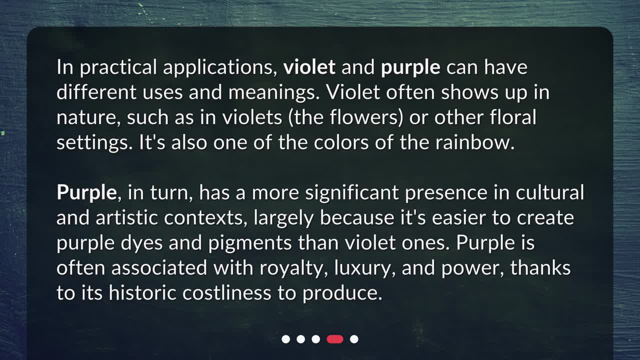 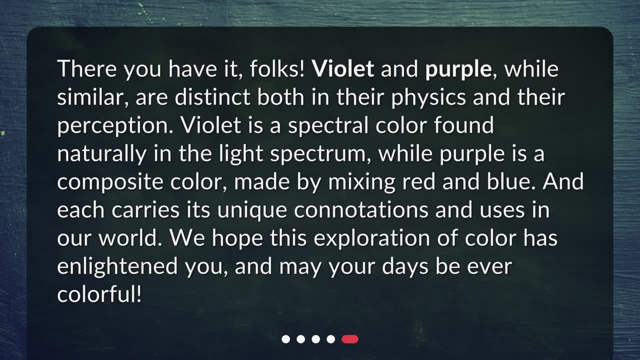 and pigments than violet ones. Purple is often associated with royalty, luxury and power, Thanks to its historic costliness to produce. violet and purple, while similar, are distinct both in their physics and their perception. Violet is a spectral color found naturally.